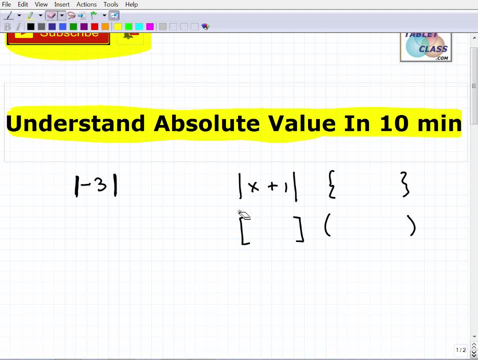 these little straight up and down vertical bars. okay, that's absolute value in mathematics. Now, just as an aside, real quick, there is something later on. it looks like this: if you're studying a little bit more advanced algebra, they have long, vertical bars are longer. This is finding the determinant of a matrix. So you don't want to confuse this with absolute value. But with that being said, let's just stick with absolute value, real basic. 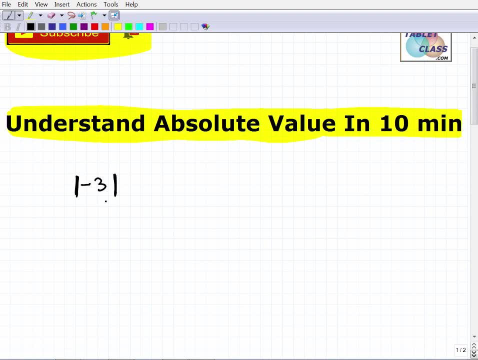 situation like this. Now what I hear a lot from students when they're first learning mathematics- you know the basic algebra level or middle school level- they'll say, oh, the absolute value of a number is the positive version of the number, right? So the absolute value: negative three. most of you would would know that that is a positive three. So what's the absolute value of positive three? Most of you out there would say, oh, that's just positive three, So you would be correct. However, you're 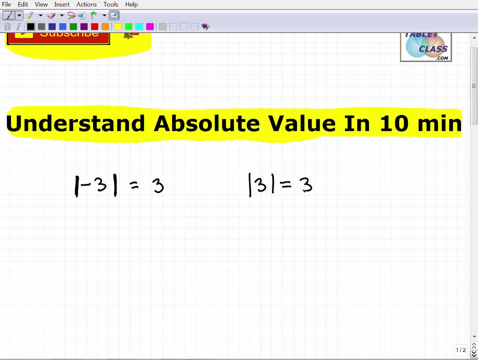 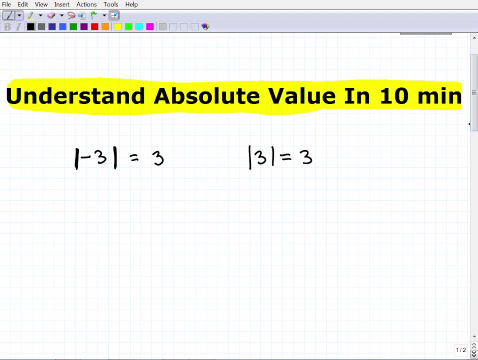 understanding the definition oftentimes is: the absolute value means the positive version of any number, whether it's positive or negative, And that's not correct. Okay, we really need to understand what the definition of absolute value is, because this is going to come into play And later different topics of absolute value. So, as you progress in your math education, you're going to be learning about absolute value, working with just the basic operation of it, And then you're going to be learning 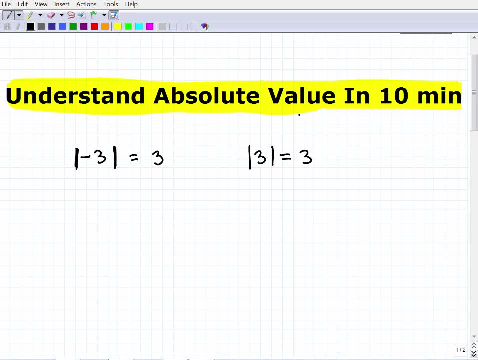 absolute value equations. I'm going to make various videos. I probably already have them on my YouTube. video certainly solve a lot of these problems, But you can study absolute value equations, absolute value inequalities, absolute value graphs and there's even some other things in there as well. So it's a big topic in algebra. let's get back to the. what we want to accomplish in this video is just understanding the essence of absolute value. So what is absolute value? Now? 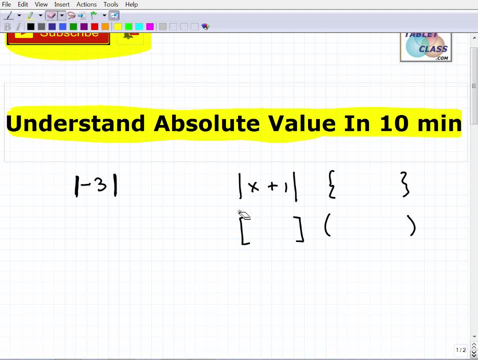 these little straight up and down vertical bars. okay, that's absolute value in mathematics. Now, just as an aside, real quick, there is something later on. it looks like this: if you're studying a little bit more advanced algebra, they have long, vertical bars are longer. This is finding the determinant of a matrix. So you don't want to confuse this with absolute value. But with that being said, let's just stick with absolute value, real basic. 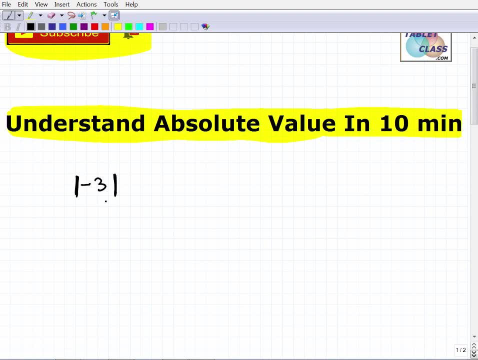 situation like this. Now what I hear a lot from students when they're first learning mathematics- you know the basic algebra level or middle school level- they'll say, oh, the absolute value of a number is the positive version of the number, right? So the absolute value: negative three. most of you would would know that that is a positive three. So what's the absolute value of positive three? Most of you out there would say, oh, that's just positive three, So you would be correct. However, you're 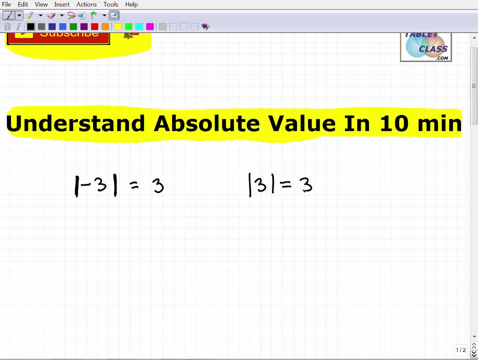 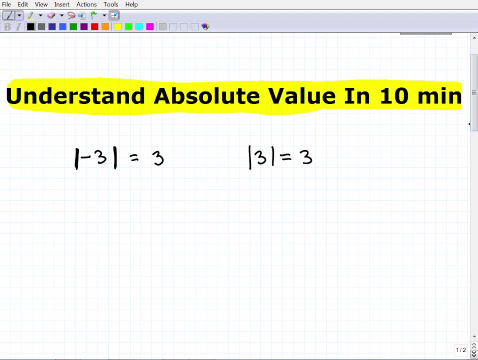 understanding the definition oftentimes is: the absolute value means the positive version of any number, whether it's positive or negative, And that's not correct. Okay, we really need to understand what the definition of absolute value is, because this is going to come into play And later different topics of absolute value. So, as you progress in your math education, you're going to be learning about absolute value, working with just the basic operation of it, And then you're going to be learning 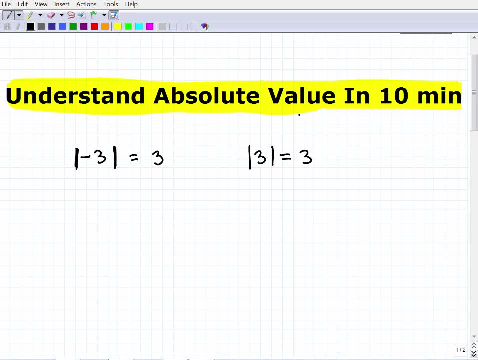 absolute value equations. I'm going to make various videos. I probably already have them on my YouTube. video certainly solve a lot of these problems, But you can study absolute value equations, absolute value inequalities, absolute value graphs and there's even some other things in there as well. So it's a big topic in algebra. let's get back to the. what we want to accomplish in this video is just understanding the essence of absolute value. So what is absolute value? Now? 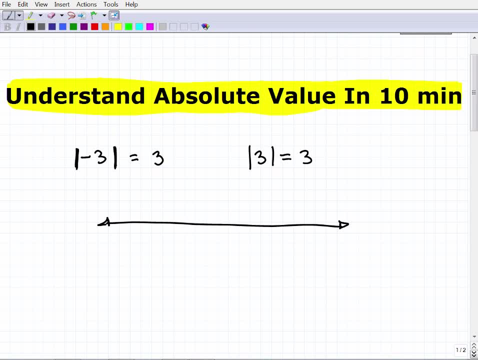 these two problems with three. I answered correctly. okay, the absolute value of negative three is a positive three. an absolute value of a positive three is a positive three. So what is absolute value? Well, absolute value is actually, technically, by definition, the distance a number is from zero on a number line. So this is a number line, number line. you've probably seen this. we really want to refer to this. 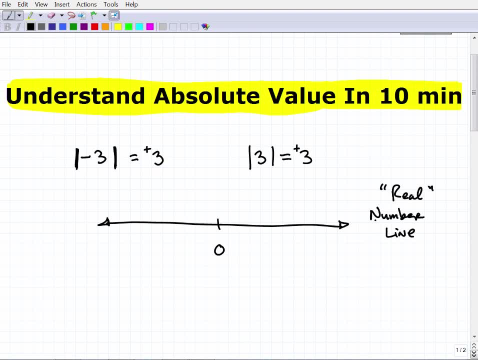 as the real number line, but that's kind of a side topic. So here we have zero in the middle, we go out 123. And as we continue to, the right, numbers get larger, right. And this way, as we go left we go, we numbers get smaller. So we have negative one, negative two, negative three. So what I'm saying here is absolute value of negative three and the absolute value of three are both positive. 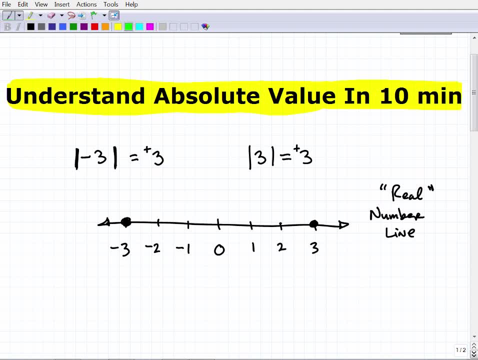 three. So what does that mean? Well, what it means is that the distance, the distance negative three is from zero- is in fact three units away. Okay, now, this is a real big point that I'm going to make: distance. distance is always measured in positive units. Okay, we kind of- there's another word out there, a little technical- says it's like displacement. 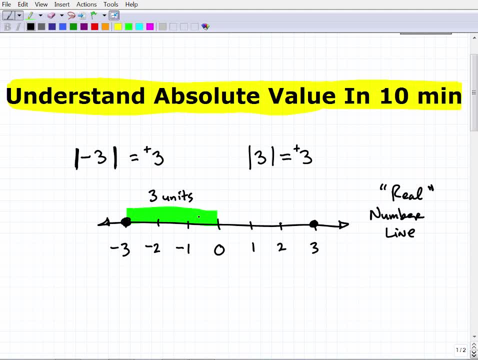 Or distance positive units. So if you had like a kind of roar and you say, hey, you know. or a tape measure said, go ahead and tell me from zero to negative three, how you know how far away is that? And you might say, well, that's three units, but your tape measure, your ruler, is not going to be saying negative units Now. likewise, three to zero is also three units away. Okay, so these are positive values. Again, distance positive units. 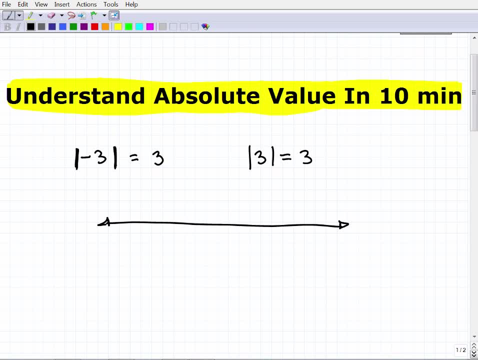 these two problems with three. I answered correctly. okay, the absolute value of negative three is a positive three. an absolute value of a positive three is a positive three. So what is absolute value? Well, absolute value is actually, technically, by definition, the distance a number is from zero on a number line. So this is a number line, number line. you've probably seen this. we really want to refer to this. 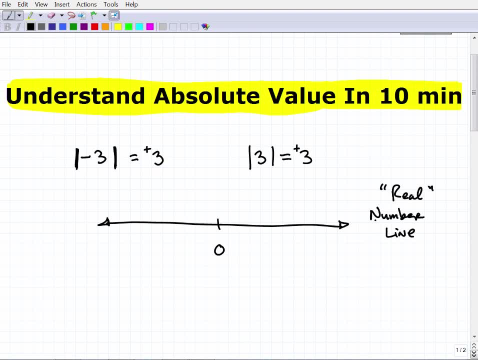 as the real number line, but that's kind of a side topic. So here we have zero in the middle, we go out 123. And as we continue to, the right, numbers get larger, right. And this way, as we go left we go, we numbers get smaller. So we have negative one, negative two, negative three. So what I'm saying here is absolute value of negative three and the absolute value of three are both positive. 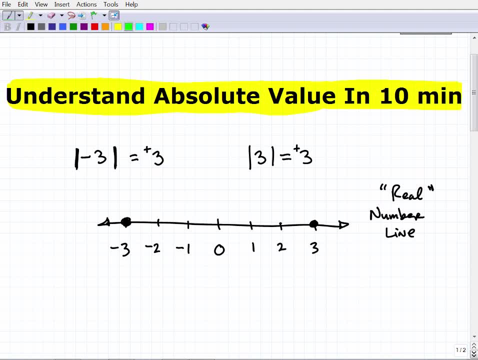 three. So what does that mean? Well, what it means is that the distance, the distance negative three is from zero- is in fact three units away. Okay, now, this is a real big point that I'm going to make: distance. distance is always measured in positive units. Okay, we kind of- there's another word out there, a little technical- says it's like displacement. 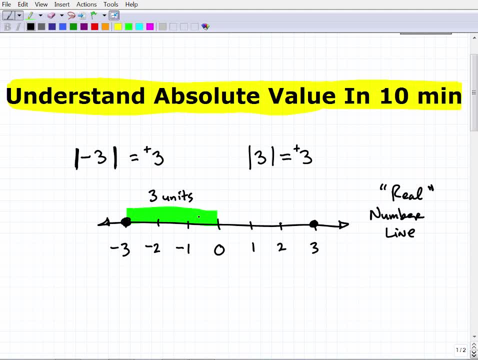 Or distance positive units. So if you had like a kind of roar and you say, hey, you know. or a tape measure said, go ahead and tell me from zero to negative three, how you know how far away is that? And you might say, well, that's three units, but your tape measure, your ruler, is not going to be saying negative units Now. likewise, three to zero is also three units away. Okay, so these are positive values. Again, distance positive units. 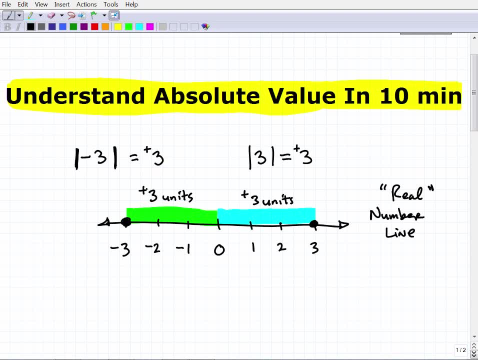 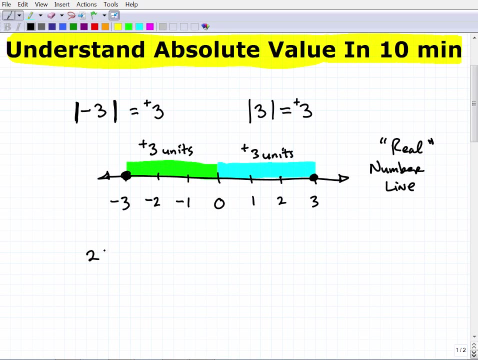 Distance is always positive. So the definition of absolute value is the distance a number is from zero on the number line. Okay, you really really need to understand that. So let's take a look at a couple basic type of problems. Let's say I have something like this: two times the absolute value negative three minus the absolute value of seven. So let's do a couple little arithmetic problems. So if you want to pause the video, 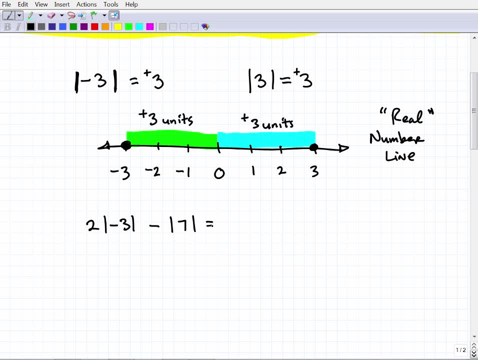 and try this yourself. you know, go right ahead. I'm going to go ahead and solve it now. So what you want to do here is let's just go ahead and take care of these absolute value functions right now. So this would be two times the absolute value. negative three is what positive three. So let's write that like this: minus the absolute value of a positive seven is simply seven. So we can just write this problem now in this manner. So we went from the absolute values into actual just numbers. Okay, so 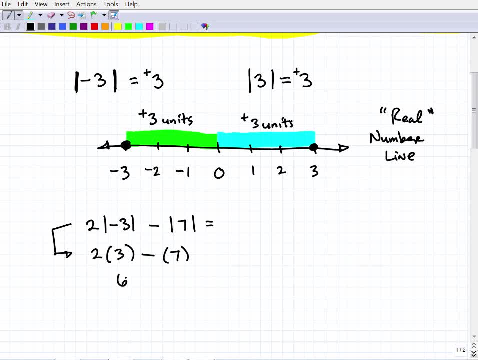 now we just finish this up. Two times three is what six, six minus seven- Hopefully you did not say one- Okay, the answer is negative one. So if you're studying absolute value at this point, you're likely have already studied positive and negative numbers, Okay, and the rules of those very, very important. A lot of students mess, you know, mess this up. So this is a real basic illustration of working with the absolute value. 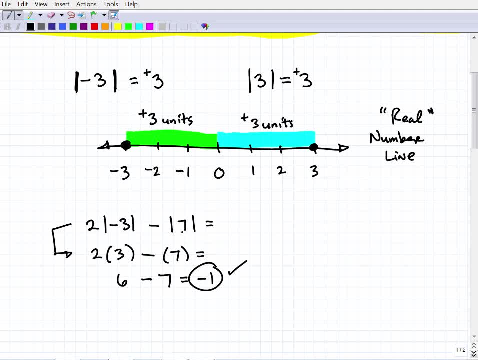 with absolute values and, and you know, basic order of operation, type of problems. Now let's take a look at something a little bit different. Okay, I'm going to write a real basic absolute value equation. So the absolute value of x is equal to three. Okay, So what is x? What? obviously x is a variable, right, So it's a variable in algebra. But what really is? 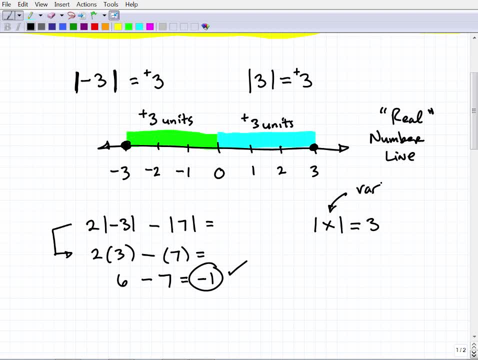 a variable. okay, here's a little pop quiz. a variable is what? what's? some number, right? so any variable- X, Y, when I just represent some number. so I want to take a look at this absolute value equation. let's do it kind of like differently. let's say the absolute value of some number, the absolute value of some number. 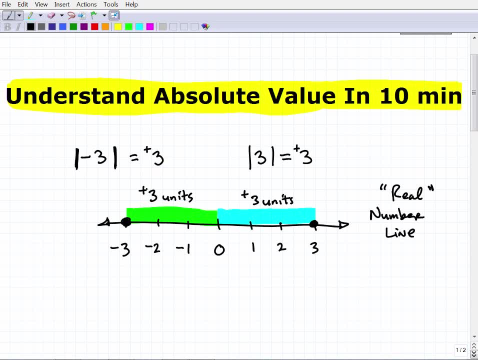 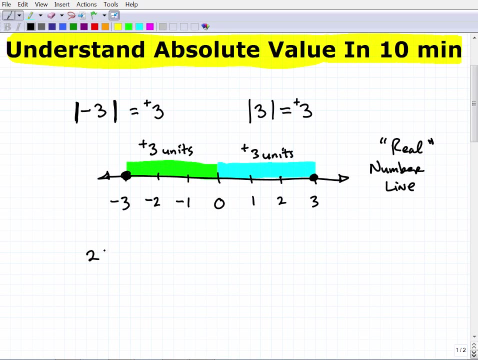 Distance is always positive. So the definition of absolute value is the distance a number is from zero on the number line. Okay, you really really need to understand that. So let's take a look at a couple basic type of problems. Let's say I have something like this: two times the absolute value negative three minus the absolute value of seven. So let's do a couple little arithmetic problems. So if you want to pause the video, 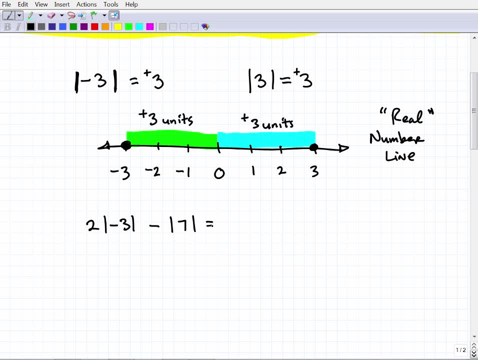 and try this yourself. you know, go right ahead. I'm going to go ahead and solve it now. So what you want to do here is let's just go ahead and take care of these absolute value functions right now. So this would be two times the absolute value. negative three is what positive three. So let's write that like this: minus the absolute value of a positive seven is simply seven. So we can just write this problem now in this manner. So we went from the absolute values into actual just numbers. Okay, so 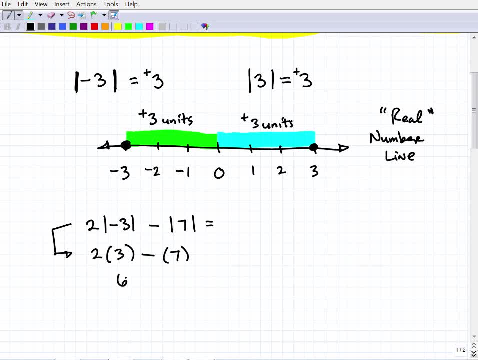 now we just finish this up. Two times three is what six, six minus seven- Hopefully you did not say one- Okay, the answer is negative one. So if you're studying absolute value at this point, you're likely have already studied positive and negative numbers, Okay, and the rules of those very, very important. A lot of students mess, you know, mess this up. So this is a real basic illustration of working with the absolute value. 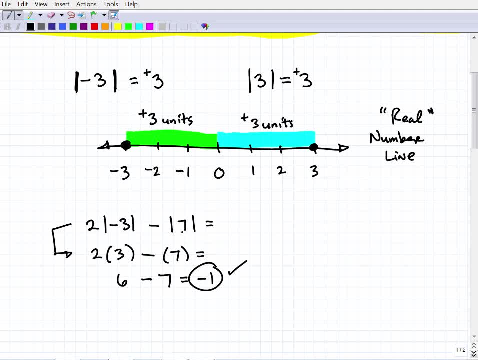 values and, and you know, basic order of operation type of problems. Now let's take a look at something a little bit different. Okay, I'm going to write a real basic absolute value equation. So the absolute value of x is equal to three. Okay, So what is x? What is obviously? x is a variable, right, So it's a variable in algebra. But what really is a variable in algebra? 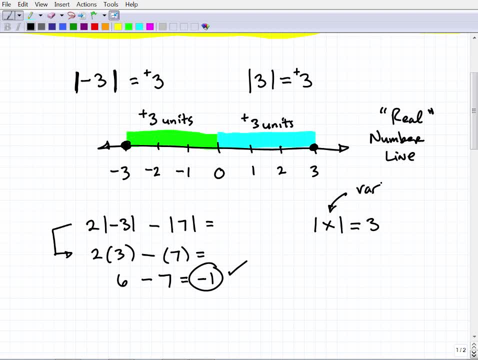 a variable. okay, here's a little pop quiz. a variable is what? what's? some number, right? so any variable- X, Y, when I just represent some number. so I want to take a look at this absolute value equation. let's do it kind of like differently. let's say the absolute value of some number, the absolute value of some number. 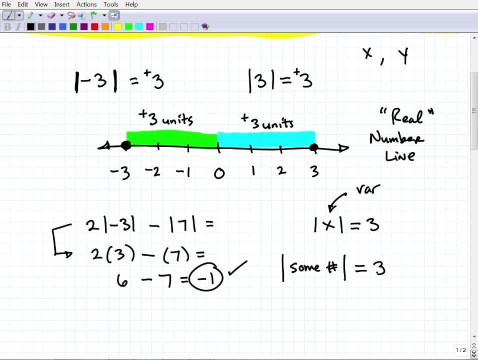 is equal to 3. okay, now, hopefully you can figure this out. if I said: hey, Sarah, you know what's I got. I got some number here and it's absolute value is equal to 3. what is that number? okay, some number is, it's absolute value is equal to three. 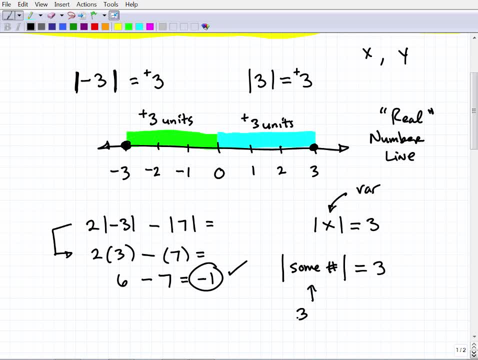 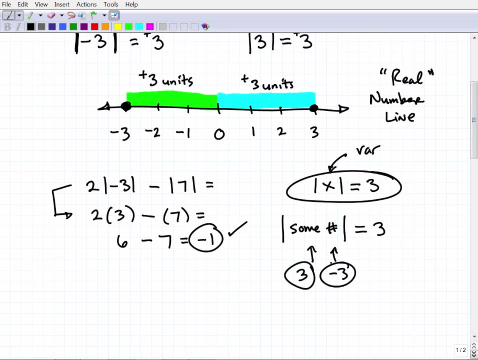 well, you would say, oh yeah, well, you're probably plugging in three, and you would be correct. but also I could find the absolute value of negative 3 and that would also be correct. okay, so the main thing that you want to remember about absolute value equations: that there's always two solutions, always. 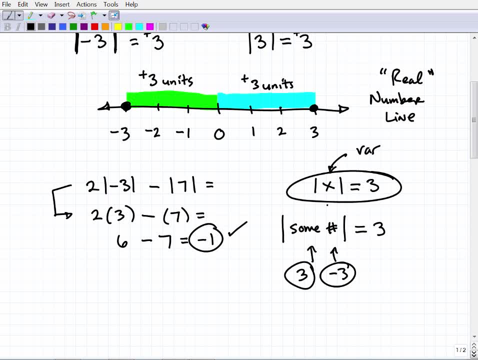 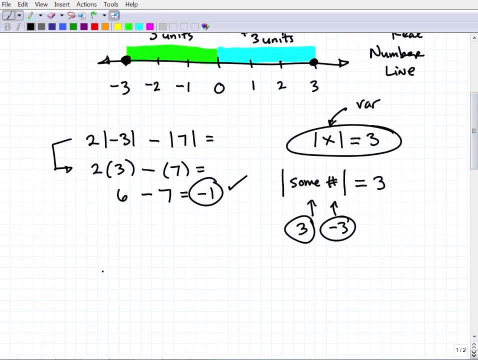 two solutions, solutions to absolute value equations. There's always going to be two solutions. Now, real quick, I'm going to just write something out: 2x plus 1, absolute value of 2x plus 1 is equal to 9, and absolute value of 2x plus 1 is less than 9.. 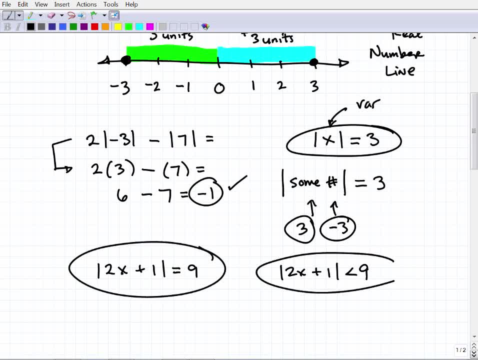 Okay, so I have an absolute value equation and an absolute value inequality. I'm not going to get into these, but I want to make a point as we wrap up this video. Both of these look pretty similar. However, the way we solve them is completely different. 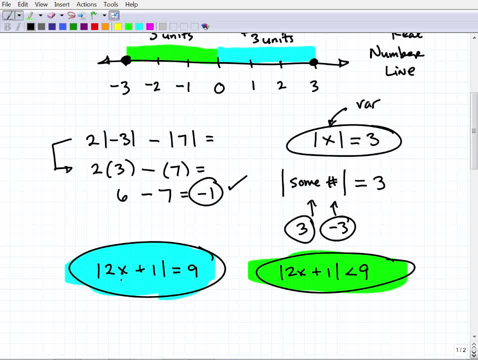 So another very common mistake is students, they'll see an absolute value equation and they'll start doing what you do for an inequality. They'll confuse this with this And that is what happens. What happens when you just try to remember math, like in a rote way. Okay, I don't know if you're familiar with that word- rote, That just means like trying to learn math by just a bunch of flashcards- not truly learning it, but just trying to remember it. 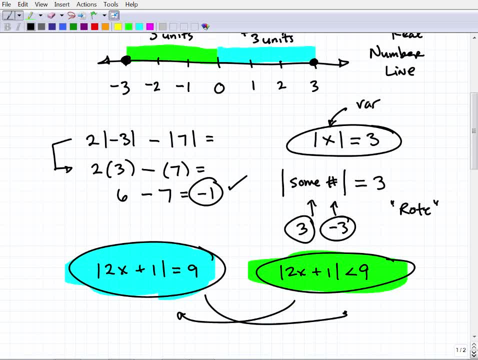 Like, okay, I'm just going to remember all this stuff. I hate it. I'm going to remember it by looking at it a million times and just hope I kind of remember it for a test. That's not the way to approach mathematics, because you're going to end up confusing things. 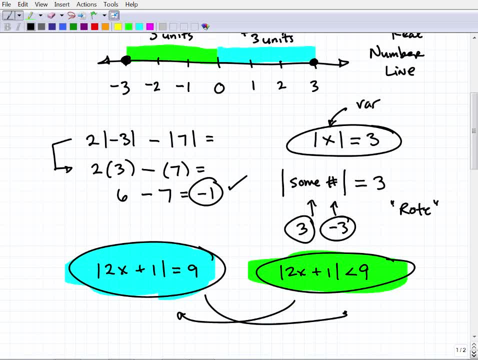 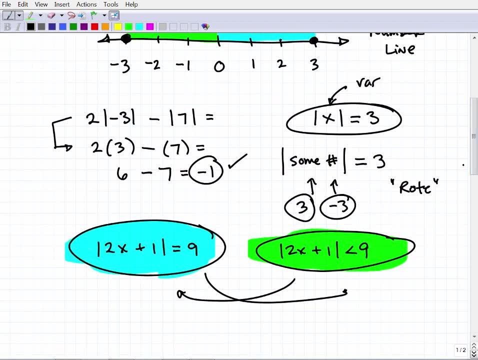 Now, how do I know this? Because I've been teaching for several years And you know- you just see the mistakes students make. So everything I'm telling you here comes from years of experience. So, as you get into these topics, you may not have started to study this yet, but you will. 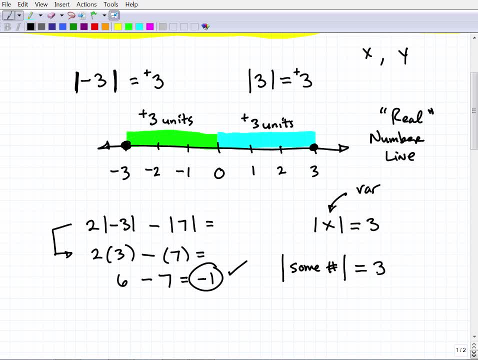 is equal to 3. okay, now, hopefully you can figure this out. if I said: hey, Sarah, you know what's I got. I got some number here and it's absolute value is equal to three. what is that number? okay, some number is, it's absolute value is equal. 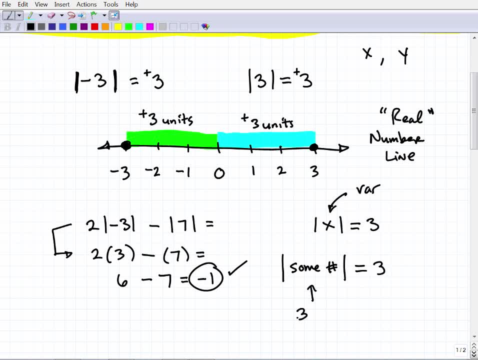 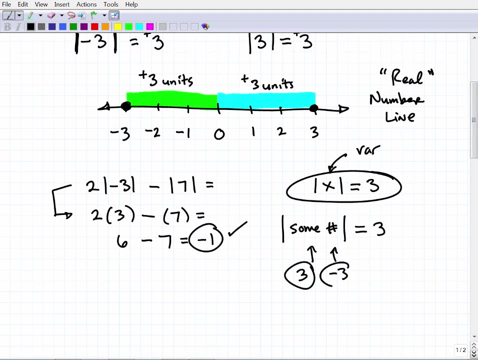 to three. well, you would say, oh yeah, well, you're probably plugging in three, and you would be correct. but also I could find the absolute value negative three and that would also be correct. okay, so the main thing that you want to remember about absolute value equations: if there's always two solutions, always two. 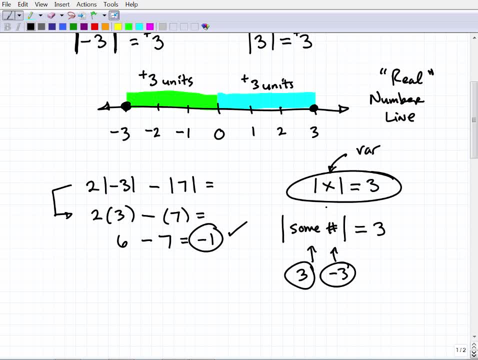 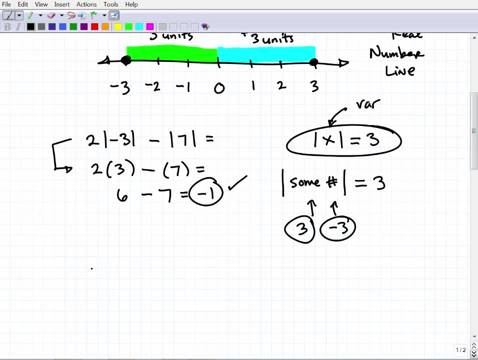 solutions: solutions to absolute value equations. There's always going to be two solutions. Now, real quick, I'm going to just write something out: 2x plus 1, absolute value of 2x plus 1 is equal to 9, and absolute value of 2x plus 1 is less than 9.. 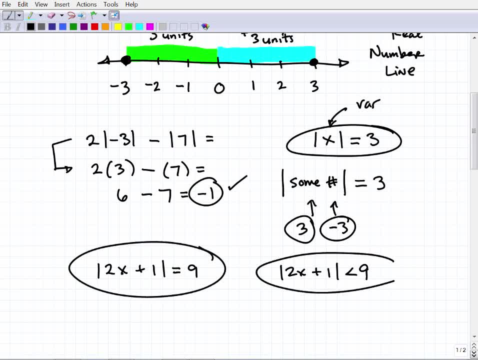 Okay, so I have an absolute value equation and an absolute value inequality. I'm not going to get into these, but I want to make a point as we wrap up this video. Both of these look pretty similar. However, the way we solve them is completely different. 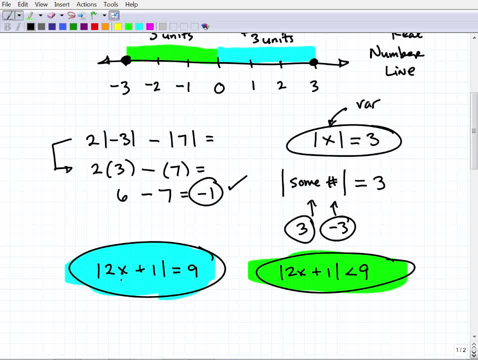 So another very common mistake is students, they'll see an absolute value equation and they'll start doing what you do for an inequality. They'll confuse this with this And that is what happens. What happens when you just try to remember math, like in a rote way. Okay, I don't know if you're familiar with that word- rote, That just means like trying to learn math by just a bunch of flashcards- not truly learning it, but just trying to remember it. 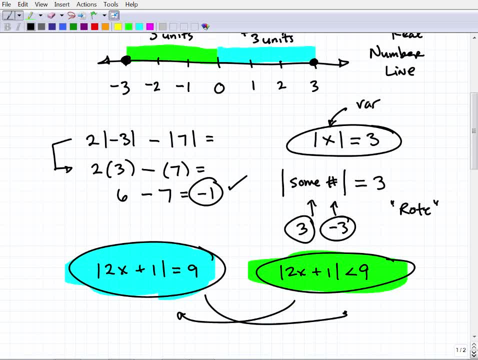 Like, okay, I'm just going to remember all this stuff. I hate it. I'm going to remember it by looking at it a million times and just hope I kind of remember it for a test. That's not the way to approach mathematics, because you're going to end up confusing things. 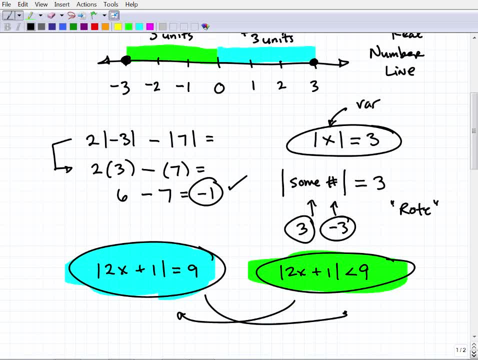 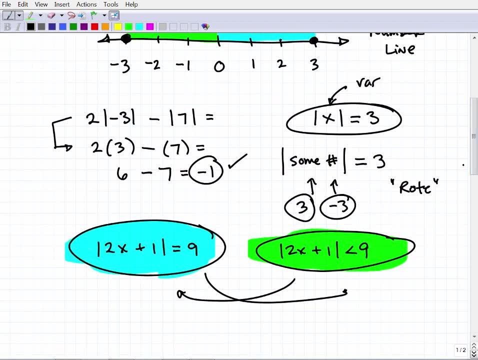 Now, how do I know this? Because I've been teaching for several years And you know- you just see the mistakes students make. So everything I'm telling you here comes from years of experience. So, as you get into these topics, you may not have started to study this yet, but you will.